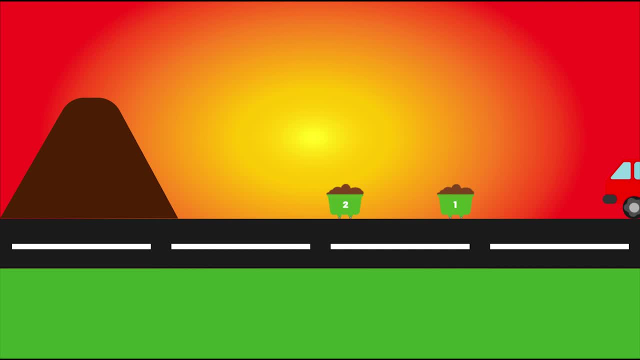 related to hauled container system. Since solid waste management involves cost in collection of waste and transportation of the waste, the involved time is also a major factor on which the cost involved can be calculated. Let's jump into the time calculation of hauled container system. 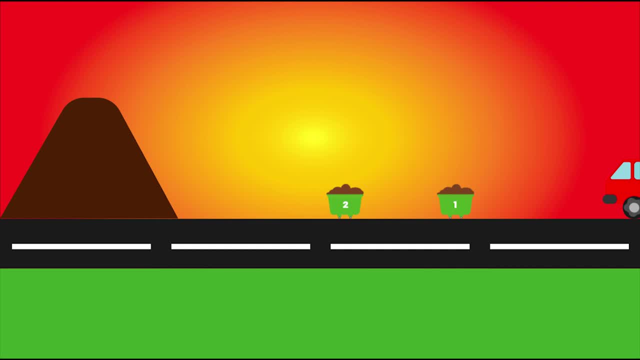 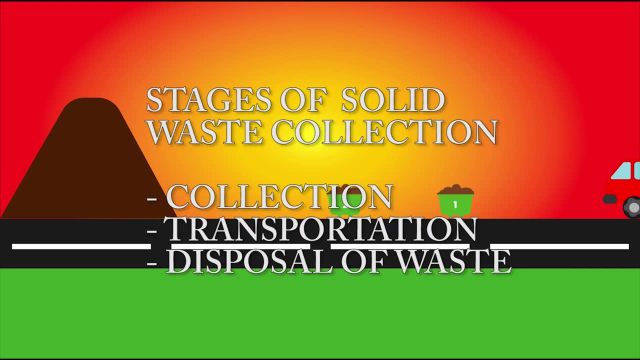 As we know, hauled container system consists the stages, such as collection, transportation and disposal of waste. Each stage has a particular time consuming activity. Now, if we pay attention here, A hauled container truck consists of two stages. The first stage contains the waste and the 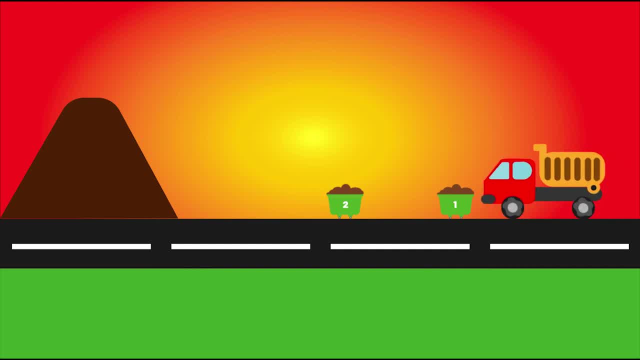 second stage includes the container travels to the container position and picks it up. The time required to pick up the container 1 filled with waste is termed as pickup time, termed as PC in short form. Now the truck travels to the disposal site for dumping. 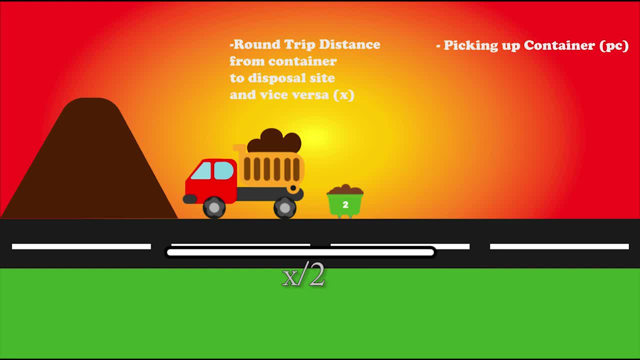 Let x by 2 be the distance from container 1 to disposal site. thus the round trip distance that is from container 1 to disposal site and from disposal site to container 1 is x. The waste truck may spend some time at disposal site waiting in line to dump the waste and 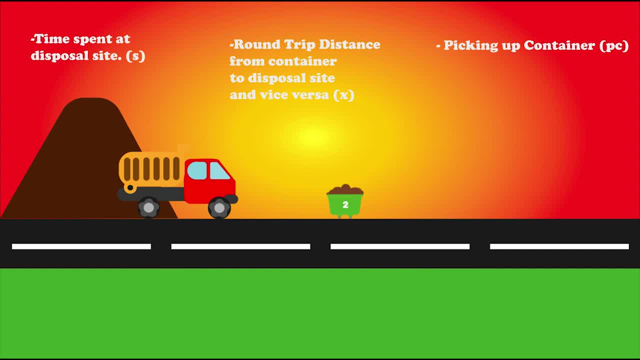 it also takes some time to dump the waste. This total time involved in the waste dump is x. The waste dump at the site is termed as at site time and is denoted as s. After dumping, the truck returns to place the container 1 in its original position. 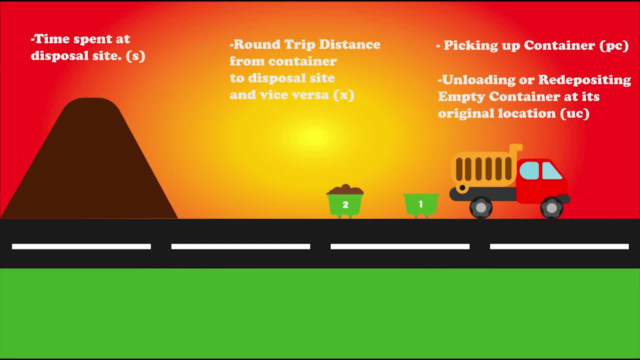 The time taken to place container 1 in its original location after coming to it is termed as unloading the container time required and is denoted as s. Now, if there are more than one waste containers, truck travels to next container. in this case, 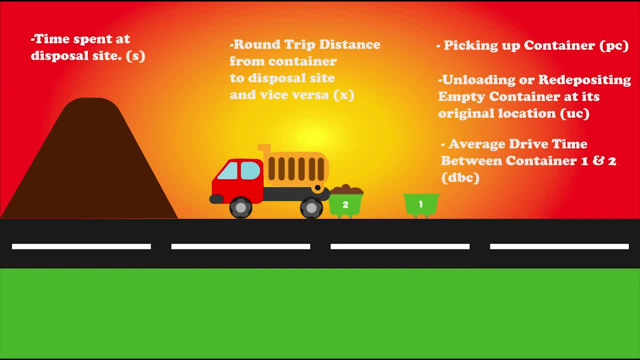 container 2 to pick up the waste. Thus, the average time taken for the truck to travel between different containers is termed as DBC, ie average time required to travel between containers. The next container that is to be picked up is container 2.. 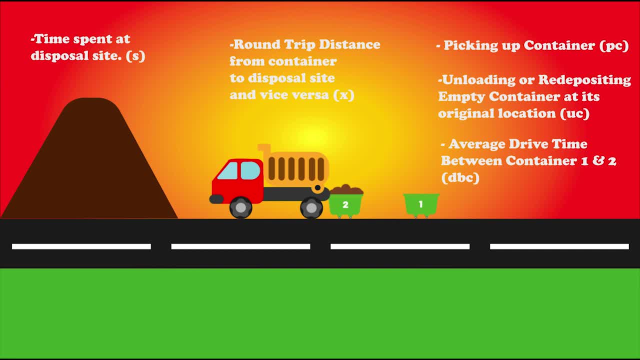 The travel time between containers is termed as dbc, ie the average time required to travel between containers, between the containers. Thus, if we look at it, the terms PC, that is picking up the waste, UC, that is unloading the waste, and DBC, that is the average time required to travel between 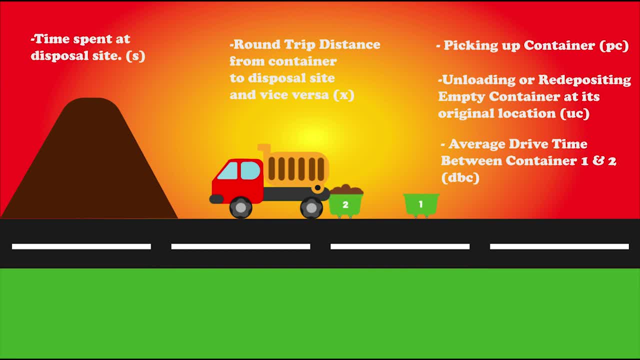 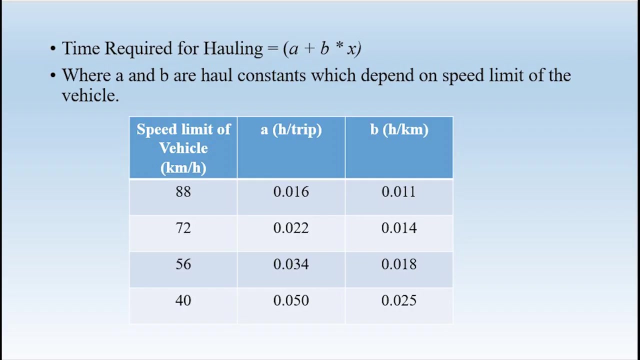 the containers will all come under and fall under the category of Pickup, which is termed as P, subscript HCS. Now if we take a look at the x distance covered by the truck, we can calculate the time required for hauling the waste, Which is A plus Bx, where A and B are the constants which depend upon the speed limit. 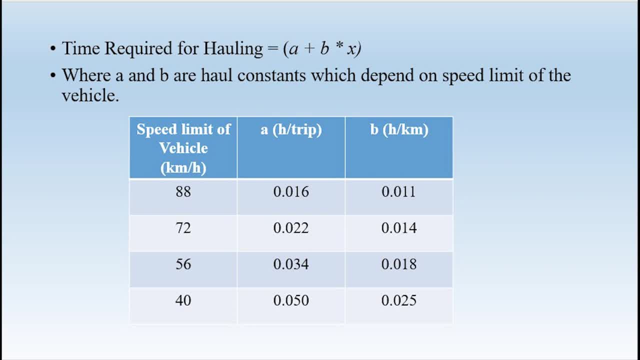 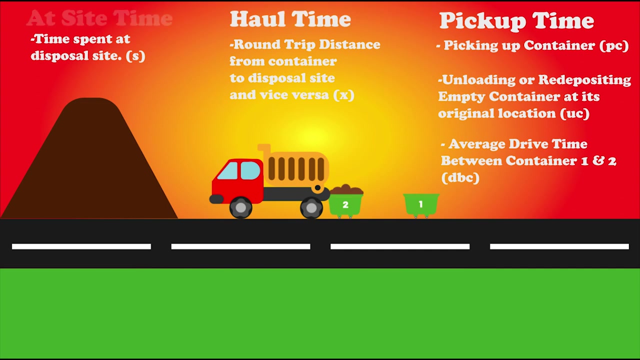 of the truck. And x, you know, as you already, it is the round trip distance covered by the truck, That is, from container to disposal site and disposal site to container. And this, termed as P, which is used in moving or moving trucks too, and which is dragged back to the side as HCS. 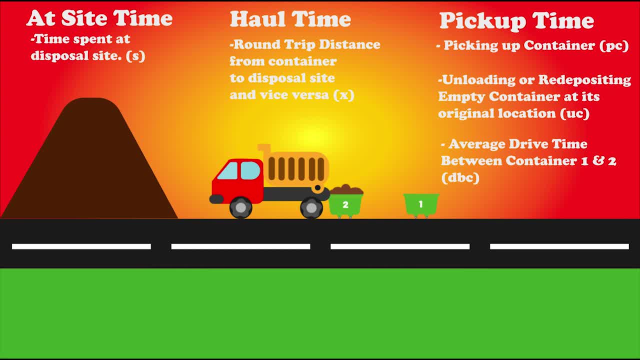 The next one is the time spent at the site. We will look at that очерly. So there is youtube and tv learning channel, mp3, facebookcom, which is google practice for AlrightyCard, the feature of Youtube, and all the activities of 93Nets. Research for. 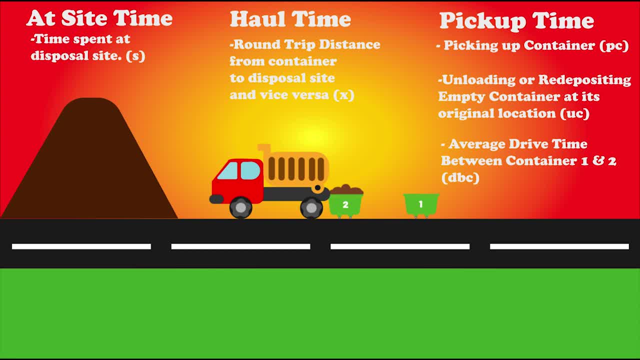 2013.. This could start as planned for 2020, to continue on, but that is what we will look. pickup time: These three combined together will give us the time required for a hauled container in a round trip. There might be also another term which.